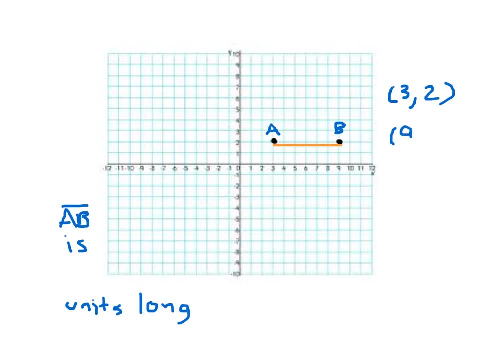 The coordinates for point B would be 9,, 2.. And remember that coordinates go x, then y. Now, the length of this line segment is determined, in this case, by subtracting 9 and 3, which are the x coordinates, Because the y coordinates are the same. 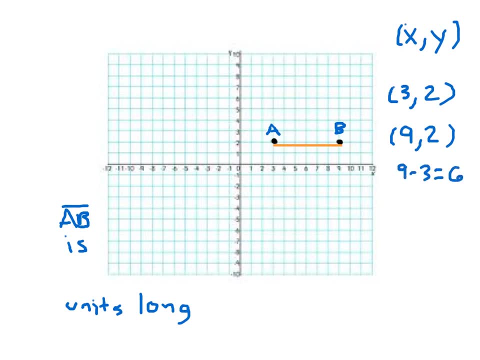 And then. so 9 minus 3 is 6.. And then, so again, we compared. since the x coordinates are the ones that are different, we compared them to find out how far apart they were: 9 minus 3, which is equal to 6.. 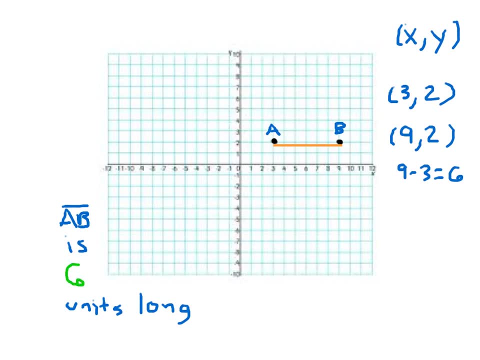 And then so we say that line segment A, B is 6 units long. So from A to B we have 1 unit away, 2 units away, 3 units away, 4,, 5, and 6 units long. 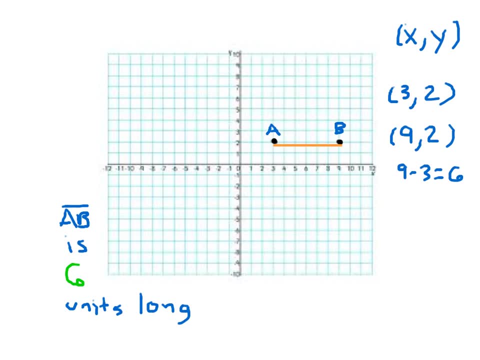 Not always will we have a graph where it is that we can count. Remember you can't count that as 1.. You have to go 1 away, which is 1,, 2,, 3,, 4,, 5, and 6 units long. 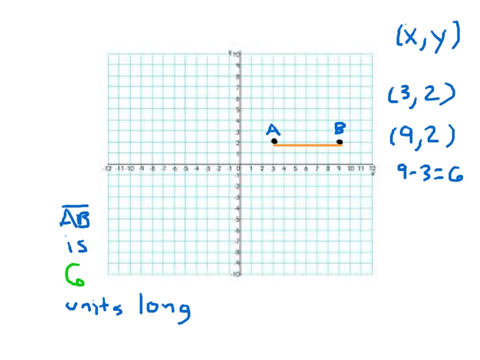 So that is a common mistake. And then, so we have 1,, 2,, 3,, 4,, 5, and 6 units long, And in this case this is a horizontal line segment because it goes from left to right. 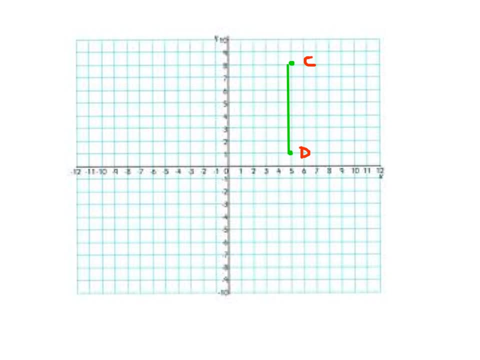 Here we're asked to find the length of line segment C, D, And then for point D, the coordinates for point D are going to be, let's see, 5, 1.. 5, 1.. The coordinates for C are 5, and then that looks like it is an 8.. 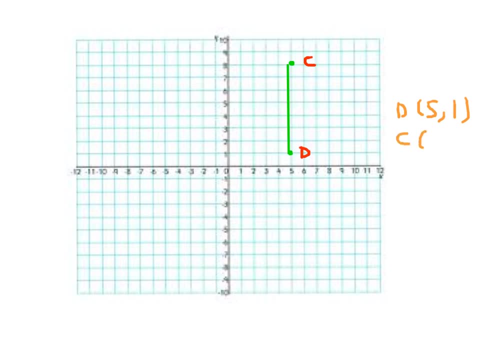 5, 8.. In this case, it is the X coordinates that are the same. So what we do is we compare the Y coordinates. We're comparing 8 with 1. How far away is 8 from 1?? So we subtract that. 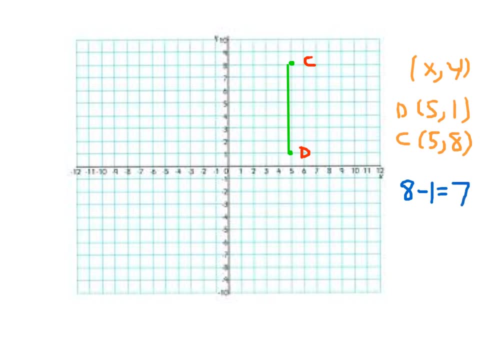 8 minus 1 is equal to 7.. And then so we say that line segment C, D is 7 units, 7 units long. Again, I can count that for you from C to D, from point C to point D. 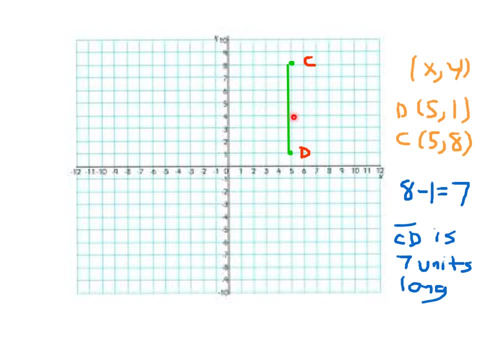 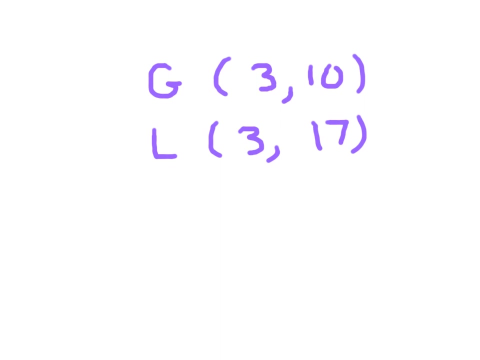 That's 1,, 2,, 3,, 4,, 5,, 6, 7 units long, 7 units long. This one is a vertical line segment. Again, not always will you have a coordinate plane to be able to just count. 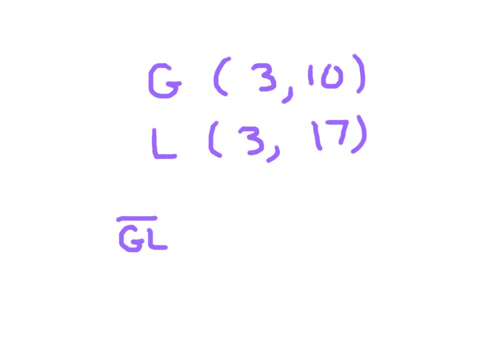 So you have to be able to figure out the lengths of line segments from just the ordered pair. In this case it is the X coordinates that are the same. So we compare the Y coordinates of these ordered pairs And to compare 17 and 10, we subtract them. 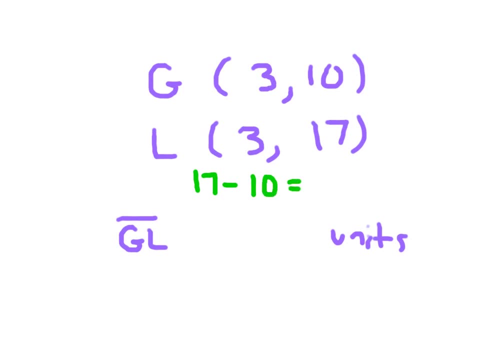 We take the larger number and subtract the smaller number away from it. 17 minus 10 is 7.. So we say that line segment GL is 7 units long. Here we have negative 2, 5,, 3, 5.. 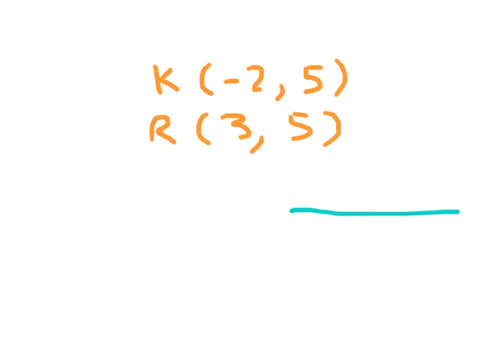 It might help us to kind of think about what it is that this one might look like in a coordinate plane. And then so remember, it's X, X axis, Y axis for negative 2, 5.. Think about here negative 2 and 5.. 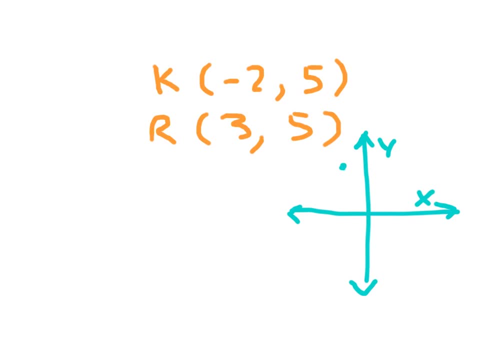 For 3, 5, we go over towards the right 3 first and then go up to get to 5. And then so that would be our line segment. So we're talking about a horizontal line segment where this for the X was negative 2.. 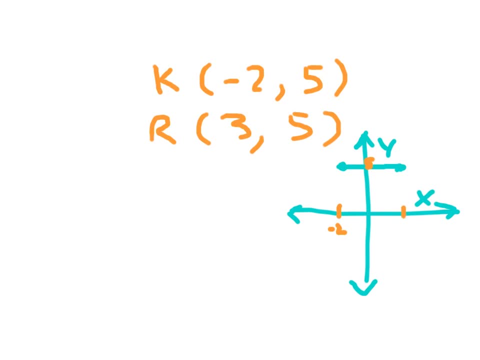 This for the Y was 5. And this right here for the X would be 3.. So really, what we're talking about is how far away it is From negative 2 to 3.. We know that's negative 2.. That would be negative 1.. 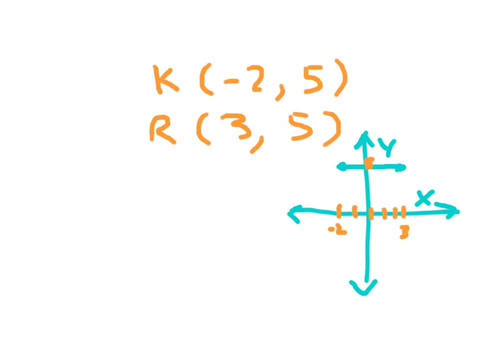 That's 0. And then we have 1 and 2. So to count from there, we would just count from there. This is 1,, 2,, 3,, 4, and 5.. So in other words, this is 5 units long. 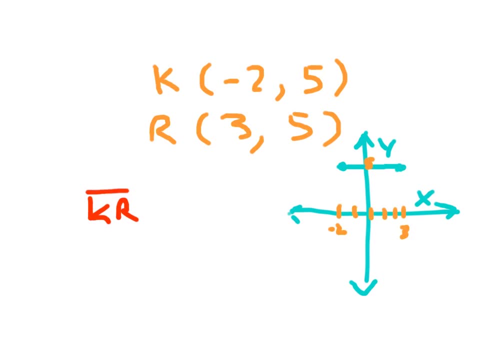 This line segment is 5 units long. Technically you can do this, The same steps that we did before, where you went. the larger number 3 minus minus 2.. 3 minus a negative is plus, So that's 3 plus 2, which equals 5.. 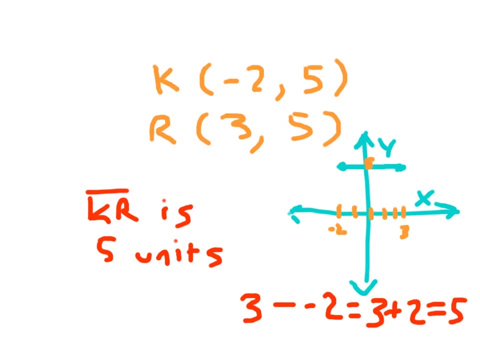 There's always more than one way to solve a problem. Line segment KR is 5 units or 5 units long, And it's because we are counting how far away negative 2 was from 3. Because the X coordinates are the ones that varied. 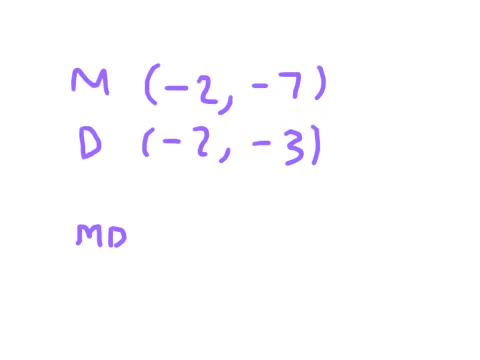 Here we have points M and points D: Negative 2, negative 7, negative 2, negative 3.. Since these two are the same- X coordinates are the same- we're going to compare the Y coordinates: Negative 7, negative 3.. 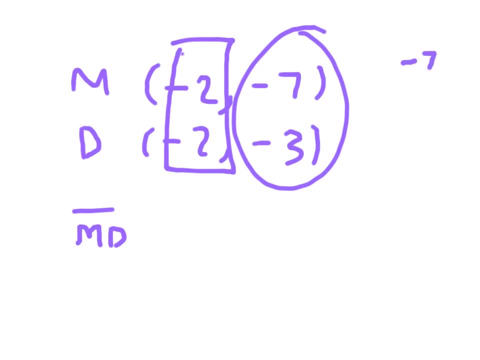 What we could do is we can actually just write those numbers out From negative 7 to negative 3.. And in this case, since we're going negative, 3 is going to be negative 3.. to be larger, we're going to go ahead and count up from negative 7, negative 6, negative 5,. 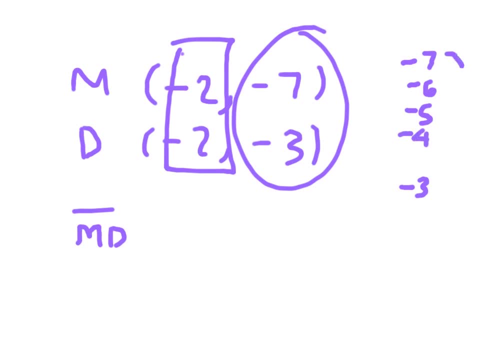 negative 4, and negative 3.. And then so, counting from there, that'd be one unit away, two units away, three units away and four units away. So line segment MD is four units long. Writing that out, it would be negative 3 minus negative 7, which is equal to negative 3 plus 7,. 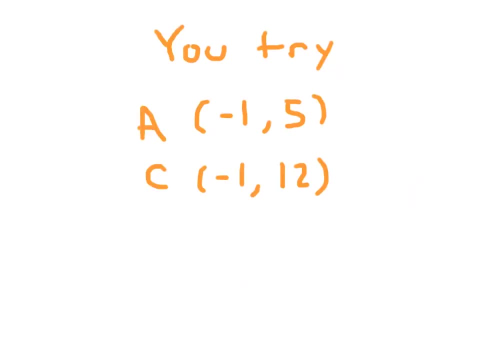 which would equal 4.. Here you try. This is points A and point C. So line segment AC is how many units long? How many units is it? Remember, in this case you're going to compare 12 and 5.. Because negative 1, the x-coordinates are the same. Write out the. 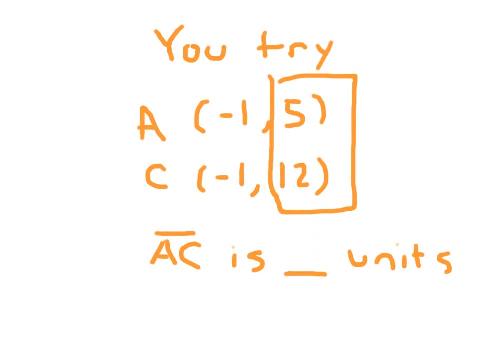 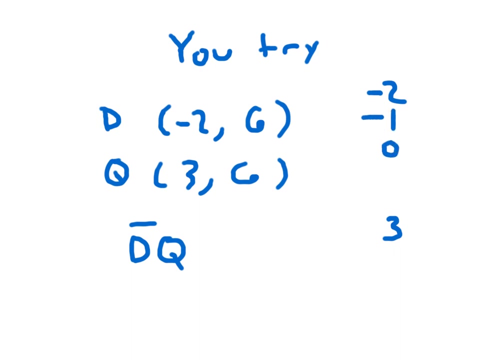 whole problem and solve it. Show that work. Did you do? 12 minus 5, which equals 7? 7 units long. Alright, hopefully you were able to solve this here, and we're only going from negative 2 to 3.. Negative 2, negative 1, 0,, 1, 2, and 3.. That's 1, 2,. 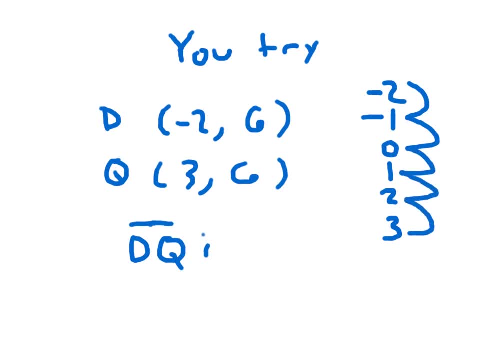 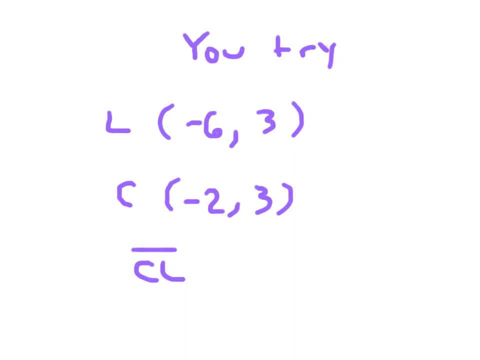 3,, 4, 5 units long. How long is line segment CL? How long is that? Think about going from negative 6 to negative 7.. Negative 2, and to count from there. Hit pause while you're trying to solve this. 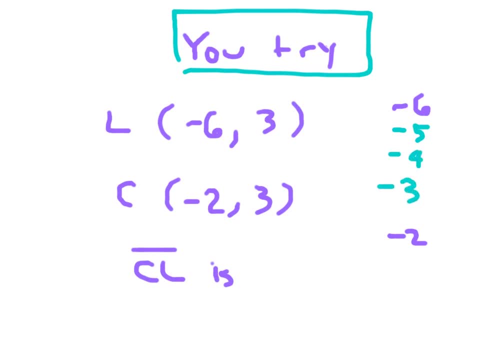 Negative 5, negative 4, negative 3,, oh, negative 2.. So that's 1,, 2,, 3, and 4.. So line segment CL is 4 units long. Writing out a number sentence for that, that would have been negative 2 minus a negative 6, which. 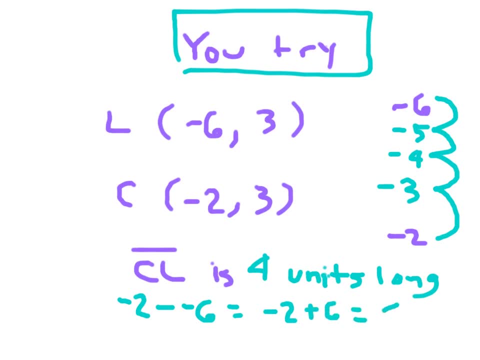 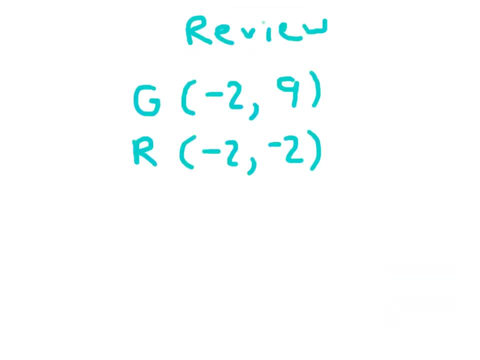 equals negative 2 plus 6,, which equals 4.. So let's go ahead and review Again. coordinates go x and then y, And in order to figure out the lengths of these vertical and horizontal line segments, you need to figure out which of those coordinates are the same for the points. 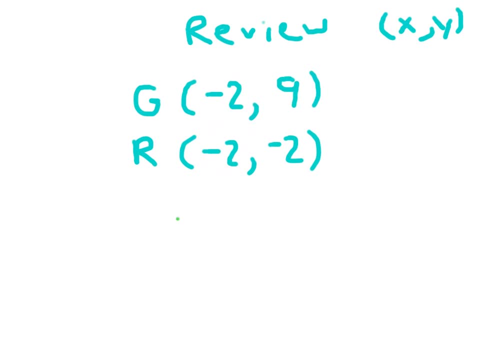 that you are looking at, And then you need to figure out which of those coordinates are also the same for the points that you are looking at, and in this case, for line segment gr, it is the x coordinate. that is the same, These x coordinates. 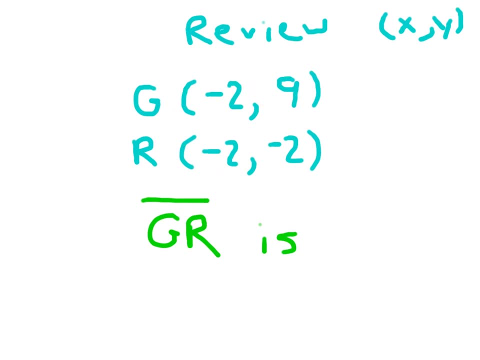 are the same. Therefore, what we're going to do is we're going to take a look at those y coordinates there and we're going to compare those. To compare them, we subtract them, or we take the larger one, which in this case would be 9, and we subtract the 2 from there, In this case, the negative 2 from.